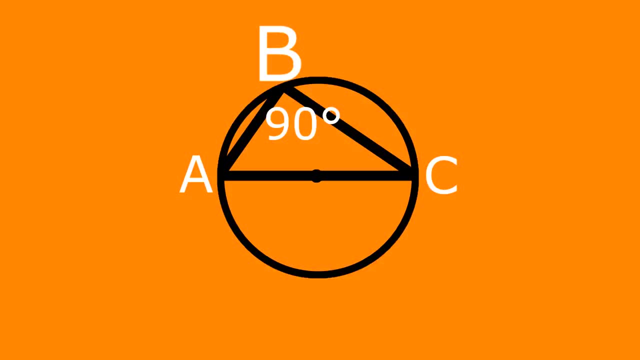 become 90 degrees. But this is no fluke. Even if we have this triangle instead, or maybe even this one, they will always be in the center. In fact, put any triangle here and it will still add up to yup, 90 degrees. 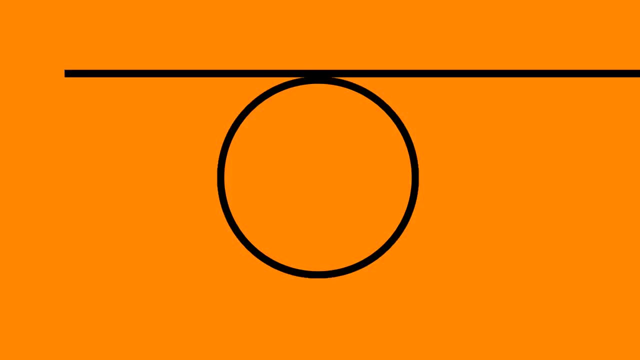 Number three: A tangent is a line that passes the outside edge of a circle. When this line is touched by the radius, that means the angle will be 90 degrees. Number four: A subtended angle is almost like our eyesight When we look at an object, our 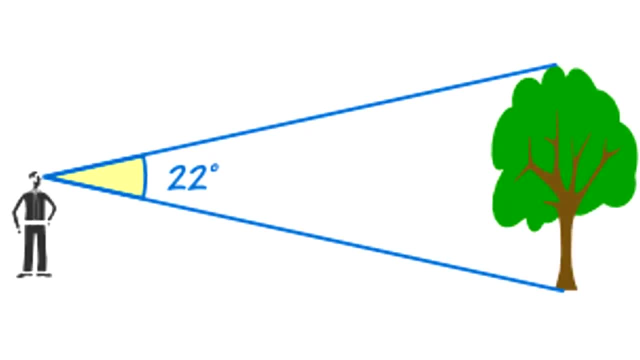 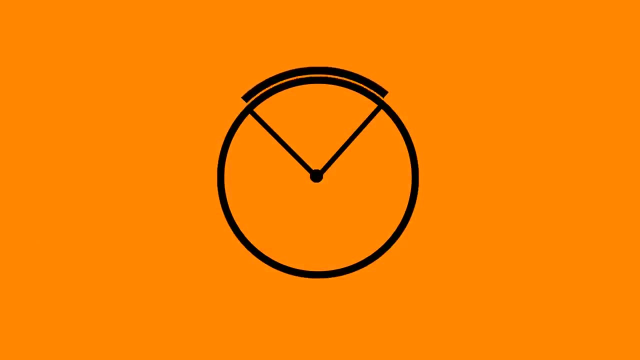 vision is focused on that. Taking this tree and this man for instance, the subtended angle is 22 degrees. The subtended angle is basically the line, arc or object opposite to the inner triangle. Number five Angles in the same segment subtended by the same arc are equal, For example, ABC. 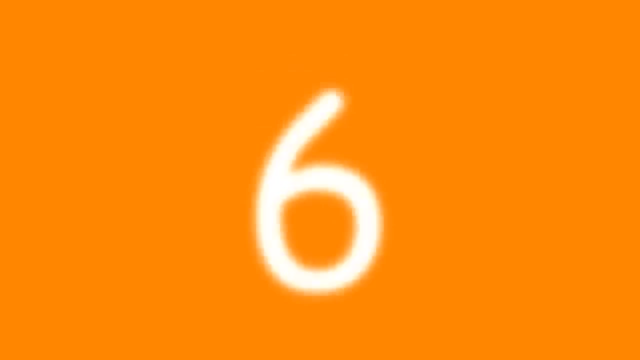 is the same as ADC. Number six: When you have an arrowhead shape inside a circle, the inner angle here is twice this angle at the circumference. Number seven: The diagram shows a cilic quadrilateral, which is a four-sided shape with all of its corners. 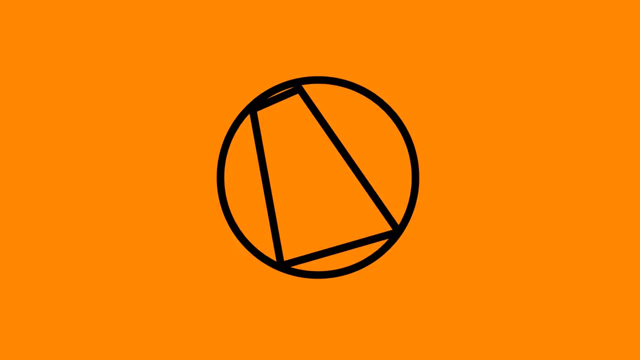 touching the circumference. What is different about this is that the opposite angles both add up to 180 degrees. So A and C would add up to 180, and B and D same thing. Number eight, Going back to the tendons, if you do not remember, go back to number three. Then the lengths. 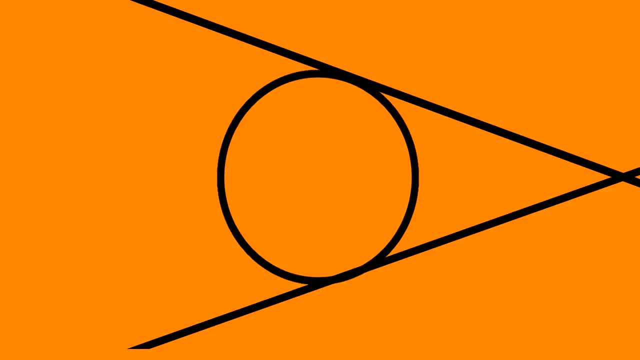 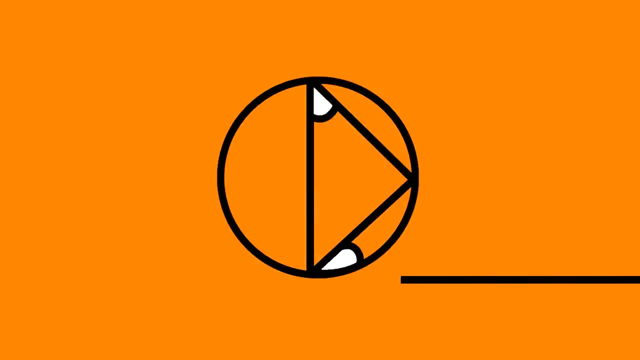 of the two tendons would equal the same amount. So explain that with a visual guide. Length AB is the same as AC. Number nine: The angle between the tangent and a chord is equal to the angle in the alternate segment. This is also known as an alternate segment theorem. 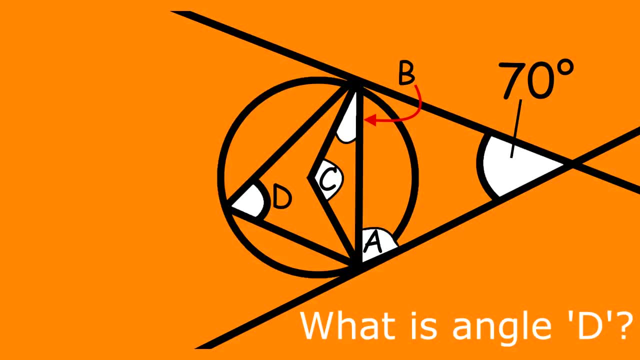 Here is a quite confusing looking sum that you are likely to get in a maths exam. Have a look at this image and have a go. Can you do it? Pause the video and see what you can get. Okay, so the sum we would do is A equals B. 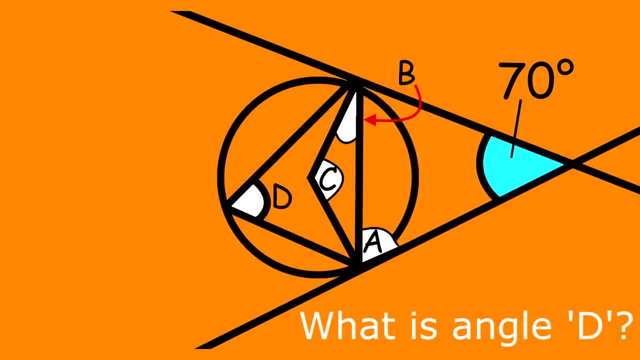 Okay, so the sum we would do is A equals B. Okay, so the sum we would do is A equals B. Okay, so the sum we would do is A equals the area that the perfect angle is. So this is: A equals 180 minus 70. Divided this all by 2 and this will equal 55 degrees. 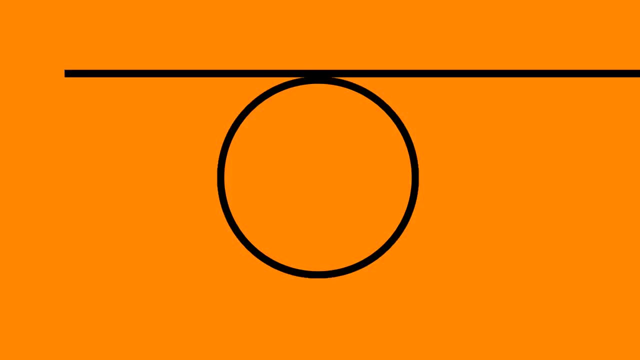 Number three: A tangent is a line that passes the outside edge of a circle. When this line is touched by the radius, that means the angle will be 90 degrees. Number four: A subtended angle is almost like our eyesight When we look at an object, our 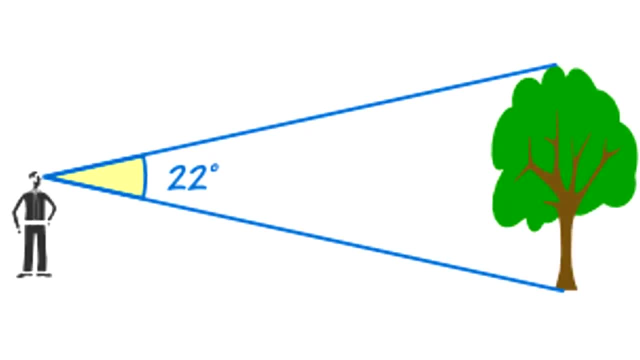 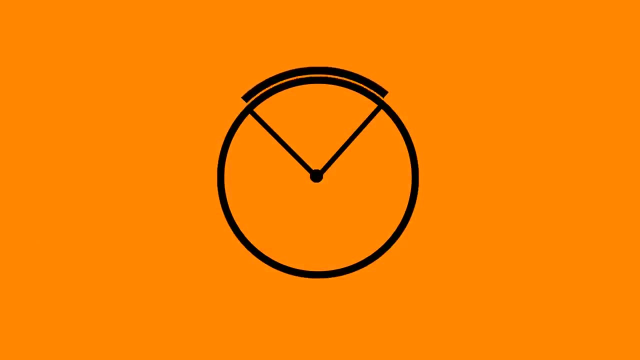 vision is focused on that. Taking this tree and this man for instance, the subtended angle is 22 degrees. The subtended angle is basically the line, arc or object opposite to the inner triangle. Number five Angles in the same segment subtended by the same arc are equal, For example, ABC. 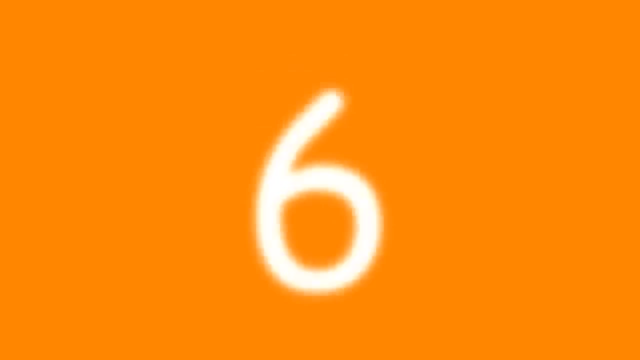 is the same as ADC. Number six: When you have an arrowhead shape inside a circle, the inner angle here is twice this angle at the circumference. Number seven: The diagram shows a cilic quadrilateral, which is a four-sided shape with all of its corners. 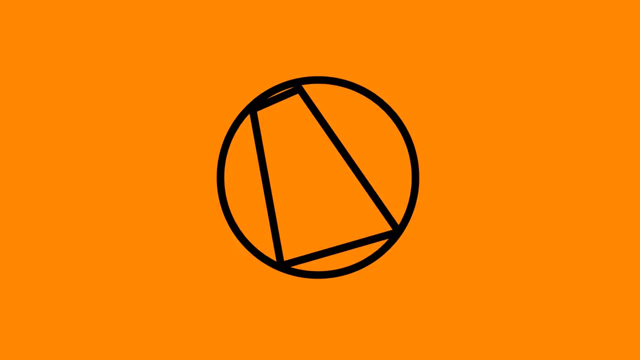 touching the circumference. What is different about this is that the opposite angles both add up to 180 degrees. So A and C would add up to 180, and B and D same thing. Number eight, Going back to the tendons, if you do not remember, go back to number three. Then the lengths. 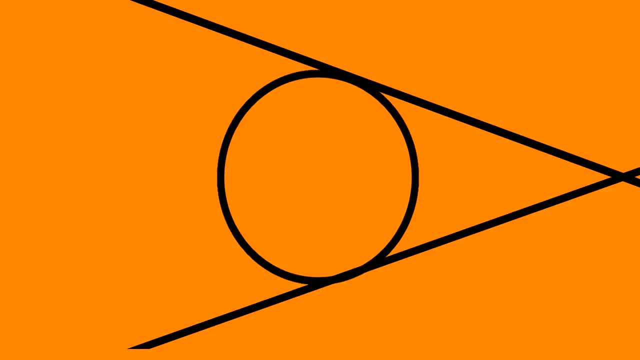 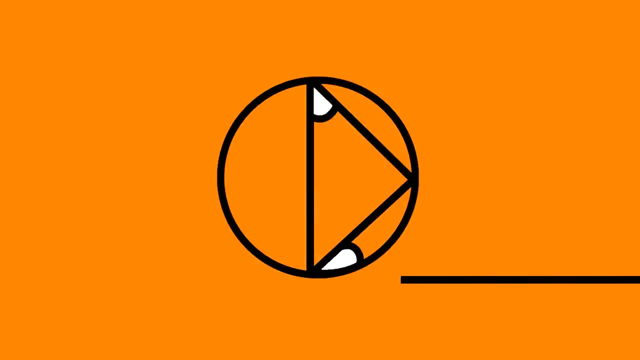 of the two tendons would equal the same amount. So explain that with a visual guide. Length AB is the same as AC. Number nine: The angle between the tangent and a chord is equal to the angle in the alternate segment. This is also known as an alternate segment theorem. 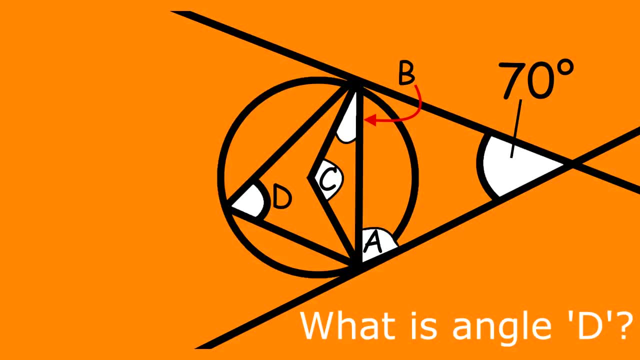 Here is a quite confusing looking sum that you are likely to get in a maths exam. Have a look at this image and have a go. Can you do it? Pause the video and see what you can get. Okay, so the sum we would do is A equals B. 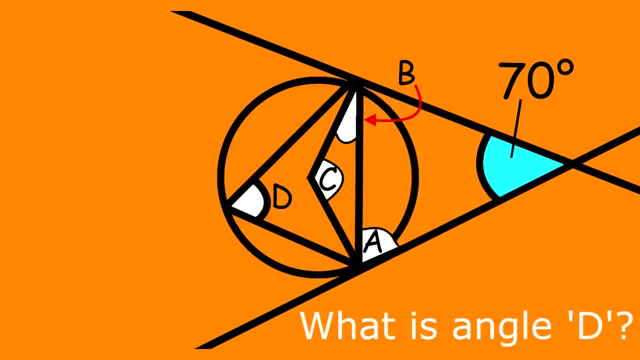 Okay, so the sum we would do is A equals B. Okay, so the sum we would do is A equals B. Okay, so the sum we would do is B equals 180 minus 70.. We divide this all by 2, and this: 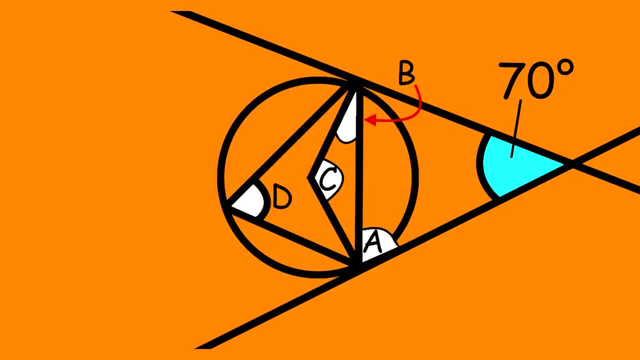 will equal 55 degrees. As some people already know, the base of isosceles' triangles will always equal. Now we get the 90 at angle B and take 55, which equals 35 degrees. How was I able to get this 90 degrees?